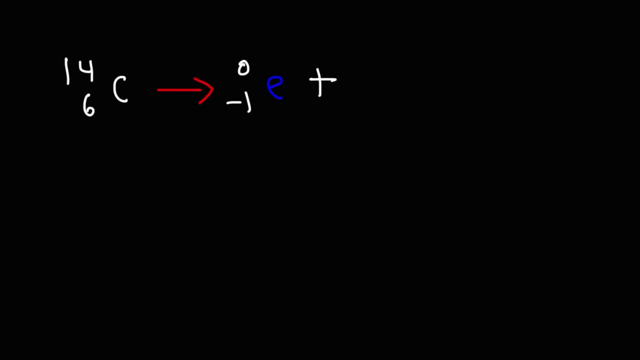 In order to do that, we need to make sure that this reaction is completely balanced. There's two numbers of interest. The 6 represents the atomic number of the element carbon, which is equal to the number of protons in this particular element, which is the same as the charge on the. 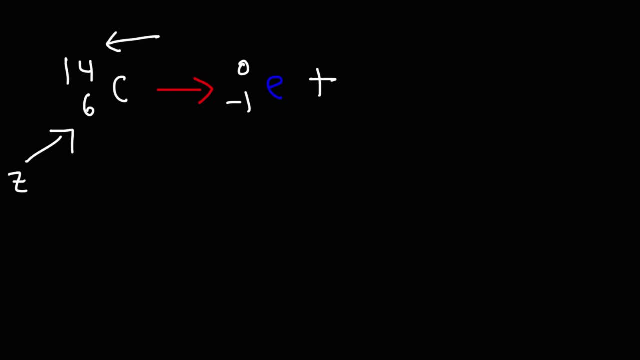 nucleus. The top number, the 14, represents the mass number of the element. It's the sum of the number of protons and neutrons. So in this element, in carbon-14, that isotope, has 6 protons, 8 neutrons. 14 minus 6 is 8.. Now, in order to balance the 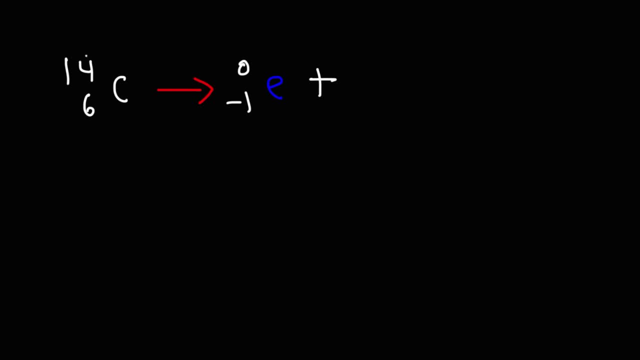 nuclear equation, we need to make sure that the mass is the same on both sides and also the total nuclear charge has to be the same. So right now this is 0, which means that we're missing a 14. Because we need a sum of 14 on the right and 14 on the left. Now, on the left side, the total nuclear 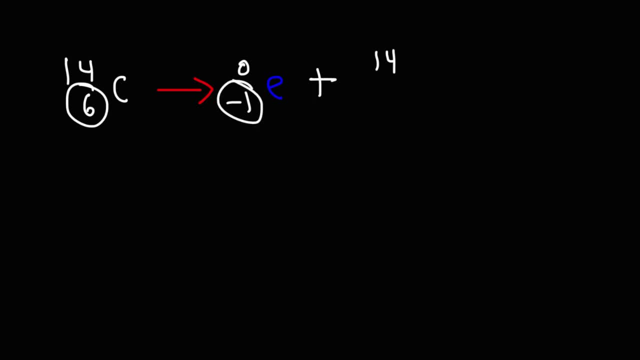 charge is 6.. On the right side it's negative 1.. So negative 1 plus what number is 6?? Now what you could do is you can write an equation. You could say: 6 is equal to negative 1 plus some missing. 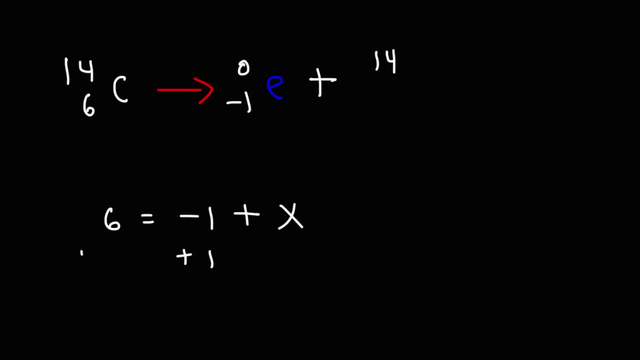 number which we can call x, and then do some algebra. In order to get x by itself, we need to add one to both sides, So x is 7.. So now that we've identified the missing atomic number, we need to identify the element and we need to use the periodic table to get the job done. So the mass numbers can vary. 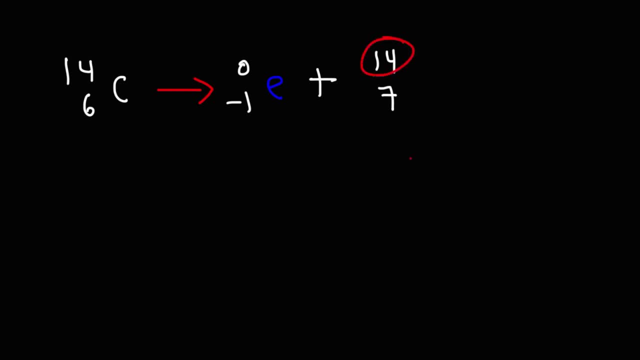 for different elements or even for the same element. However, the atomic number always identifies the element. So, using the periodic table, what element has an atomic number of 7?? There's only one, And this is nitrogen. So that's how you can identify the missing elements: by looking at the. 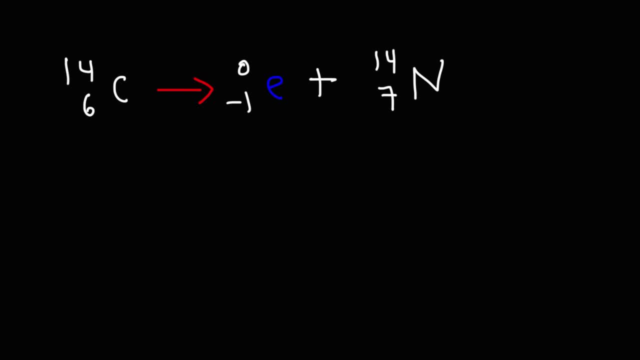 atomic number. And now the equation is balanced. We can see that the mass numbers are the same on both sides- It's 14 on both sides- and the nuclear charge is also the same. It's 6 on the left and it's a total of 6 on the right. Negative 1 plus 7 is 6.. So that's how you can balance a nuclear. 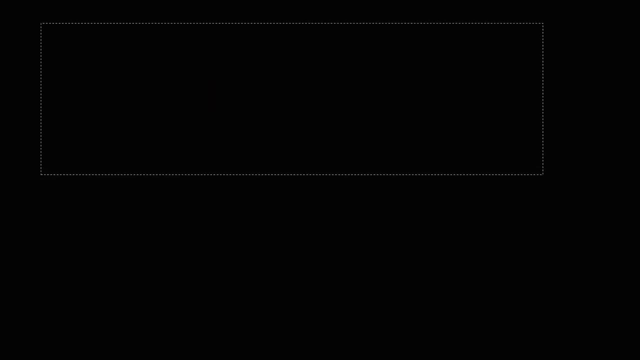 equation. Now let's get rid of that. Here's another example: Nitrogen-14 is bombarded with neutrons in the upper atmosphere and, as a result, it produces hydrogen and some missing element. What is the missing element that we need to put there to? 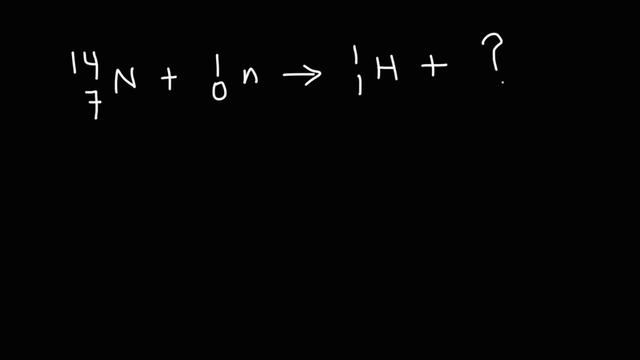 balance this nuclear equation? Go ahead and try this problem. Feel free to pause the video if you want to. So first let's write an equation starting with the mass numbers. So let's put M for mass numbers. So on the left side we have: 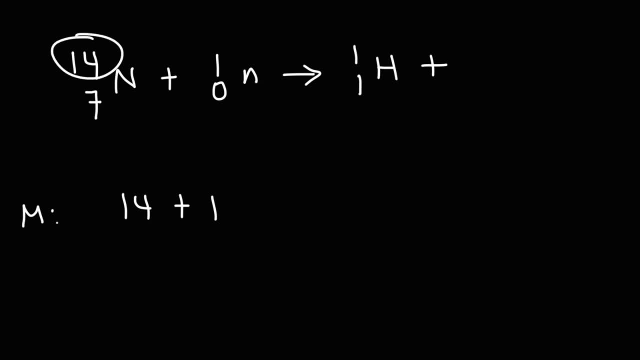 14 plus 1.. And that equals, on the right side, 1 plus some number. Let's call this y and let's call this x, And we'll call it 0. Do the same here from the bottom left, and then we're going to put 14, and that is 1, and that equals 1.. Now, considering we're halfway through, 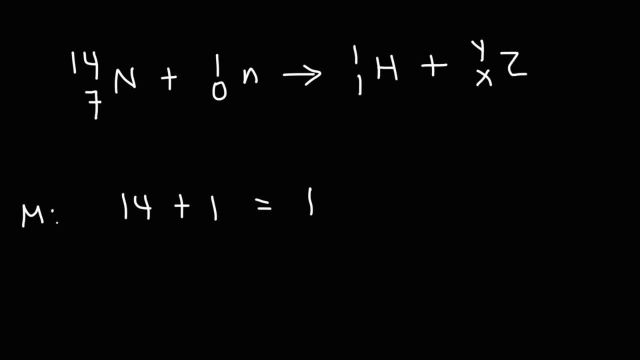 And we'll call the element. actually let's use a for this, because that's, let's make this m. I'm going through different letters here: m is for mass number, z is for atomic number and we'll say a is the element. 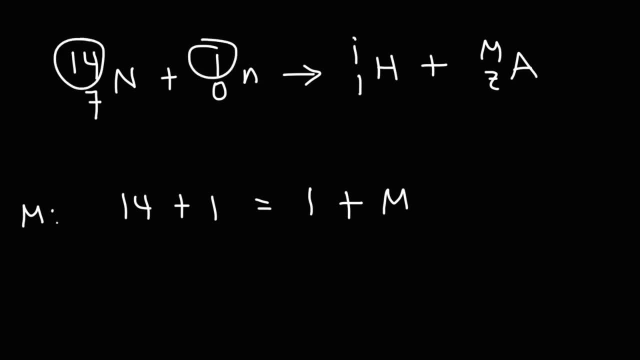 So this is going to be 1 plus m. So we have: 14 plus 1 is equal to 1 plus m. Now let's solve for m. Note that if we subtract 1 from both sides, these two will cancel and we'll get that m is equal to 14.. 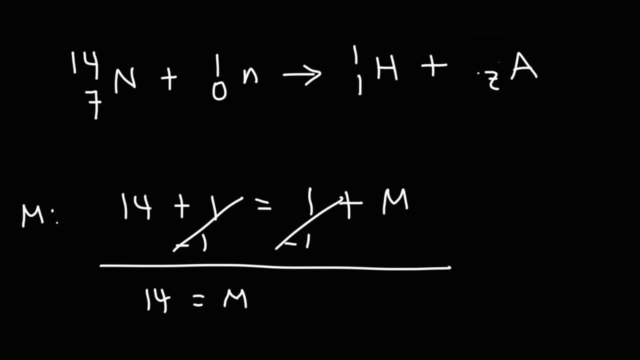 So let's replace m with that. Now let's calculate the atomic number z. So on the left, if we focus on the bottom numbers, we have 7 plus 0, and that's equal to 1 plus z. So trying to get z by itself, if we subtract both sides by 1, we can see that z is 6.. 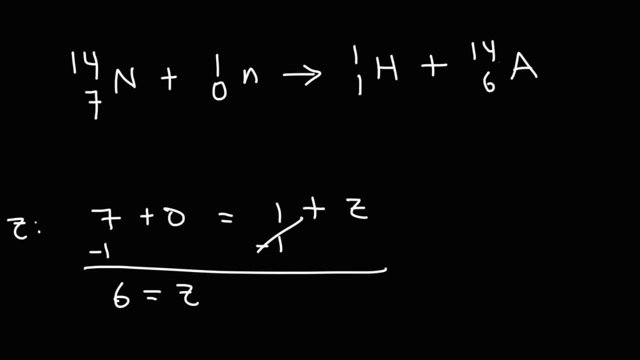 And the element with an atomic number of 6, we know this to be carbon. So when nitrogen-14 in the atmosphere is bombarded by neutrons in space, it produces hydrogen and it regenerates the carbon-14 isotope. 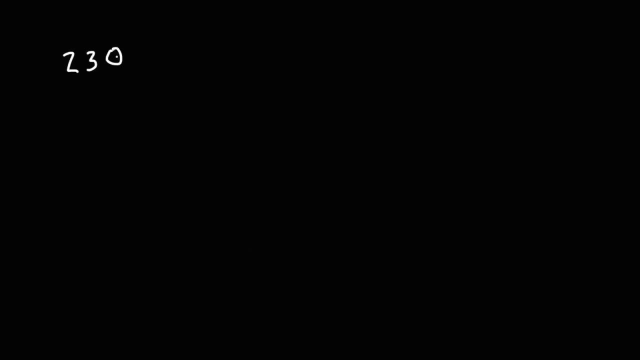 Now let's look at the hydrogen-14 isotope. Now let's work on some more examples. So next we have thorium-230, and this particular element undergoes alpha decay. So an alpha particle is basically a helium nucleus. Go ahead and identify the missing element. 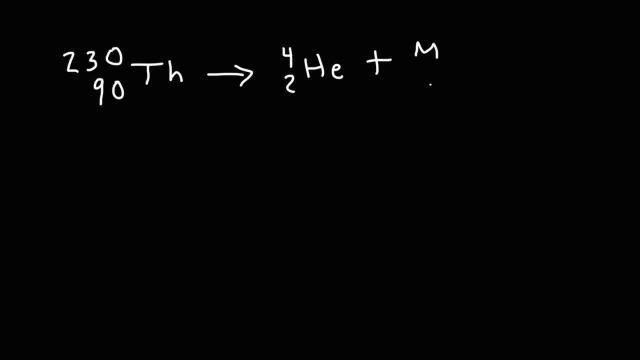 Calculate the mass and the atomic number of the missing element and then identify that element. So once again we have z And let's write an equation. So we have: 230 is equal to 4 plus m. looking at the numbers on top. 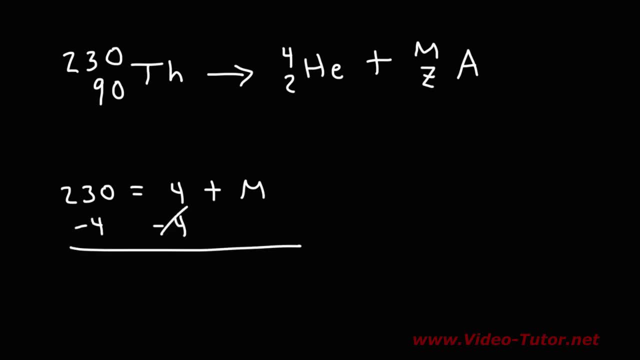 So to solve for m, we're going to subtract both sides by 4.. Thus the mass of the missing element is 226.. Now let's use the numbers on the bottom, That is the nuclear charge or the atomic numbers. So 90 is equal to 2 plus z. 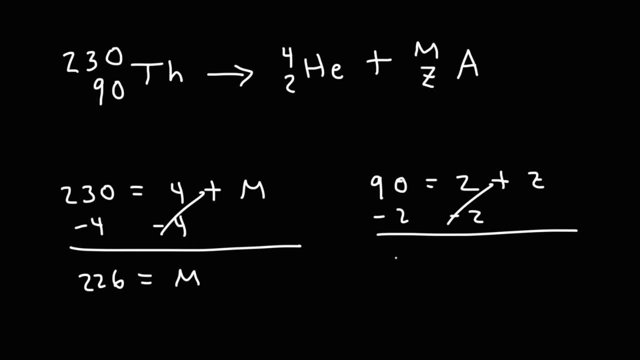 Subtracting both sides by 2, we get that z is equal to 8.. So now let's get rid of this. So our missing element has a mass of 226 and an atomic number of 88. So what element, according to the periodic table, has an atomic number of 88?? 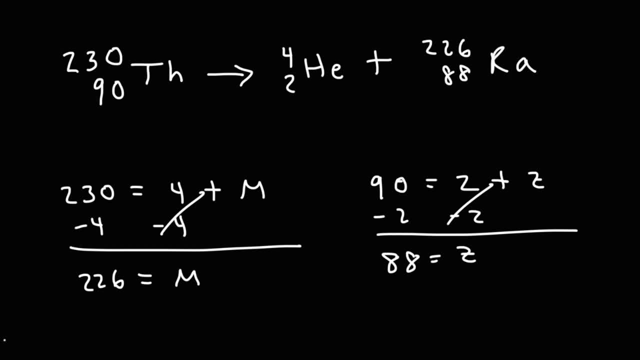 This element is Ra radium. So that's how we can balance this particular nuclear equation and, at the same time, identify the missing element. Here's another example: Mercury 201, undergoes electron capture. That is where the nucleus captures an inner core electron. 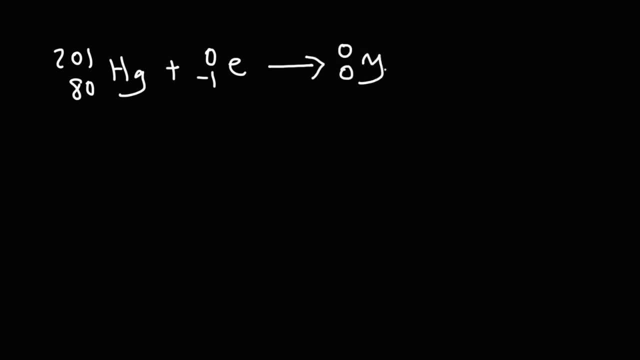 And it produces a gamma particle plus a missing element. What is the missing element? So just by looking at this, we can see that m is going to be 201, because here we have 0.. So we know that the mass of the missing element is 201. 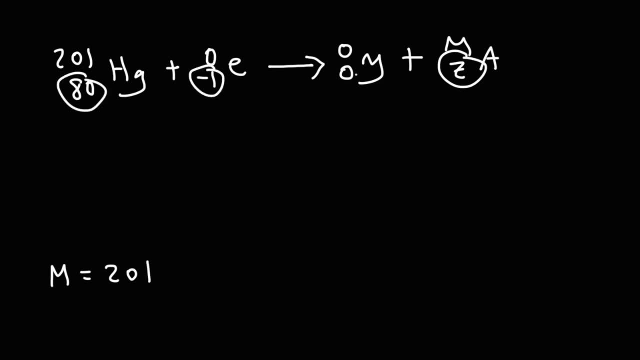 And z. we can clearly see that z is the sum of these numbers, because the 0 is not going to change anything. So 80 plus a negative 1 is 79.. So the missing element has a mass of 201, an atomic number of 79.. 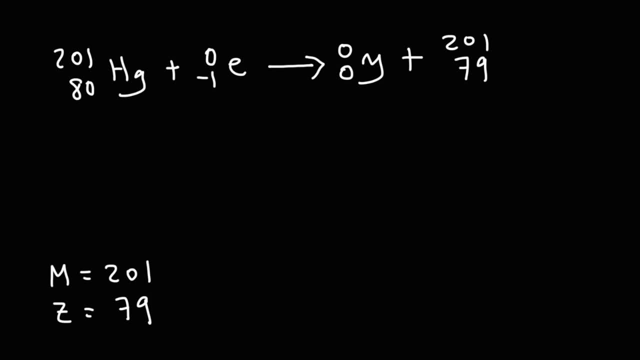 And now, using the periodic table, we can identify what element has an atomic number of 79. And this is gold. So when mercury 201, undergoes electron capture, it turns into gold 201.. What about this example? 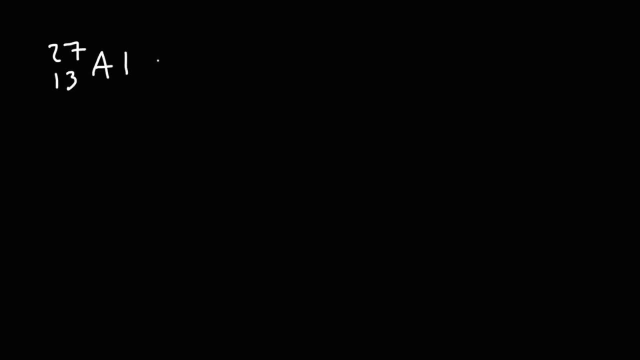 Aluminum 27, is bombarded with an alpha particle And it produces a neutron and a missing element. Go ahead and work on that example. So, starting with the numbers on top, we see that 27 plus 4 is equal to 1 plus m. 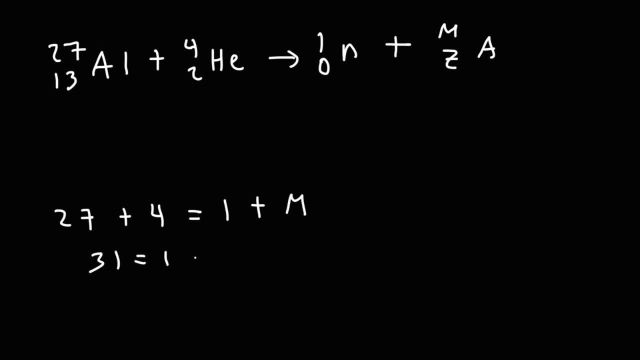 So adding 27 and 4, we get 31.. And then subtracting 1 from both sides, we can see that m is 30. And this is a missing element. So we can see that 27 plus 4 is equal to 1 plus m. 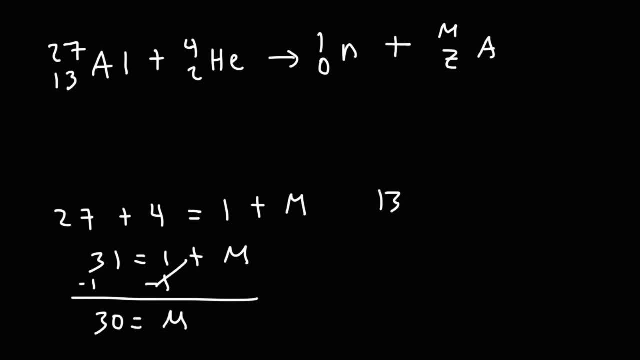 So that's the missing element in this example. Now, focusing on the numbers on the bottom, we have: 13 plus 2 is equal to 0 plus z. 0 plus z is just z. 13 plus 2 is 15.. 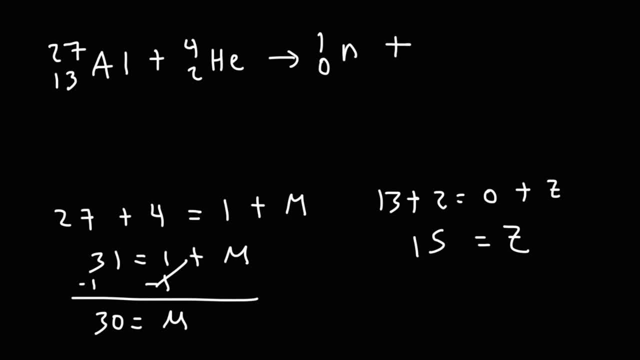 So the atomic number is 15.. So we have a mass of 30, an atomic number of 15, and the element that corresponds to a nuclear charge of 15 is phosphorus. So that's the missing element in this example. Now let's work on one more example. 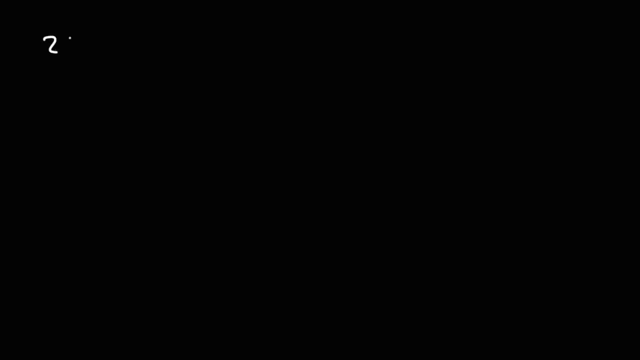 One more practice problem. Let's say we have uranium-238.. And it's bombarded with carbon atoms And in this process it generates 6 neutron particles plus the missing element. What is the missing element in this case? So let's put m, z and a.